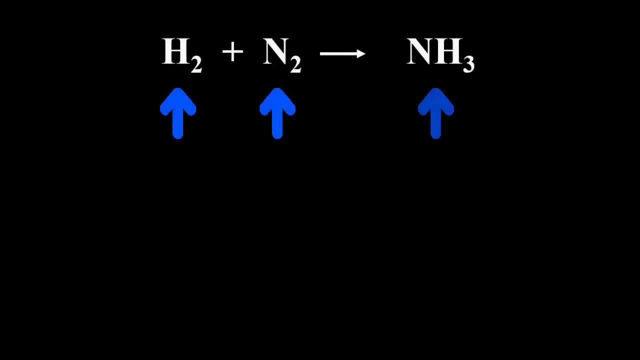 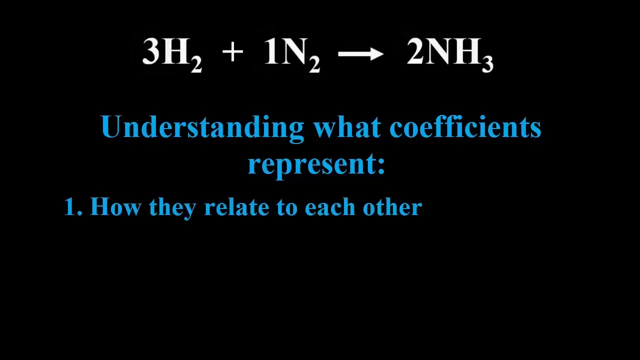 reaction, Hydrogen reacting with nitrogen to produce ammonia. It is not balanced, so we'll have to add some coefficients, And mastering stoichiometry requires an understanding of what the coefficients represent, how they relate to each other, what information can they give us, especially regarding molar amounts and how to manipulate them mathematically. 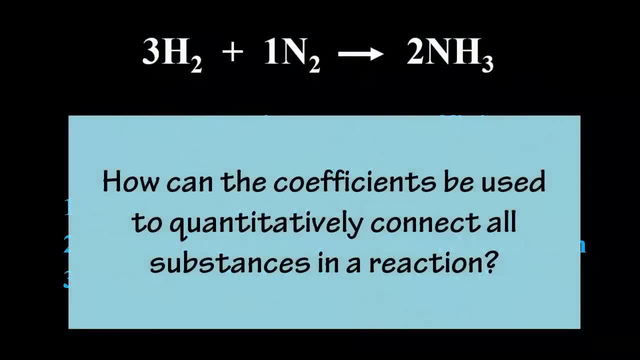 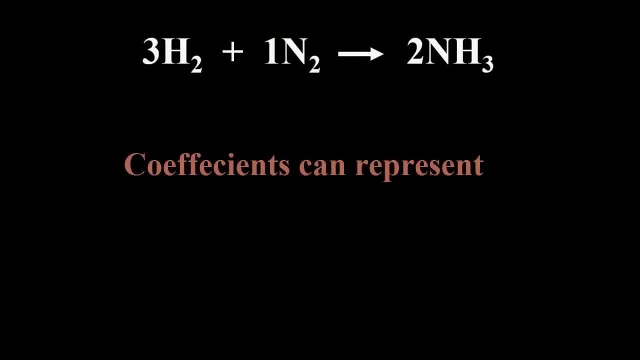 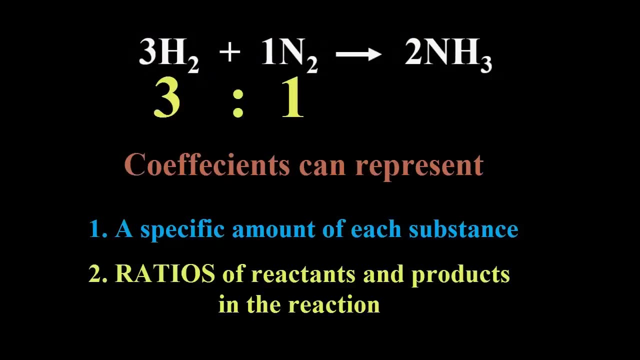 So, in other words, how can the coefficients be used to quantitatively connect all of the components in the chemical equation to each other? So we can look at coefficients as representing either a specific amount of something, an amount of particles, or as ratios of reactants and products in the reaction. 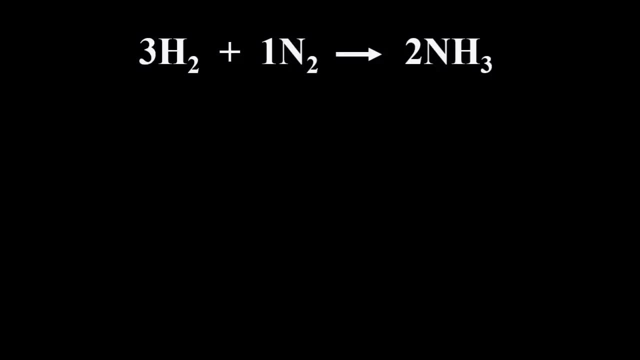 To really understand how stoichiometry works, we have to really understand what those coefficients are actually telling us. If they are referring to a specific amount of particles, that would tell us how many particles are reacting and how many particles will be produced, For example, the way the reaction 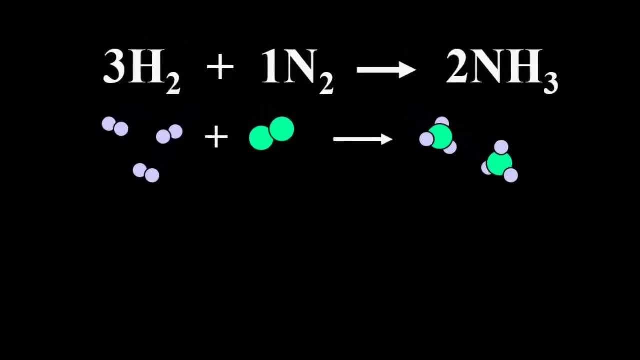 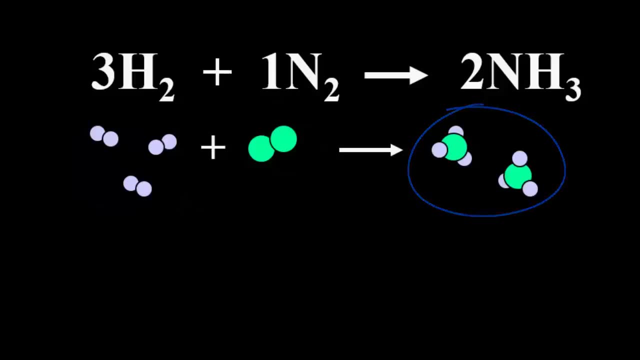 is written. as we're looking at it right here, we would have three hydrogen molecules reacting with one nitrogen molecule and that produces two ammonia molecules. So let's see how that works. The three hydrogens collide with one nitrogen. Everything is broken apart and reformed as two ammonia molecules. but in our every day, 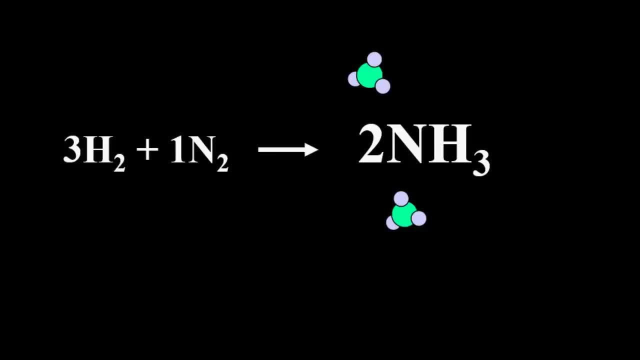 world. we are working with massive amounts of particles, and so what the coefficients can actually tell us are simply the ratios of what's going on in the chemical reaction. For example, if we have six hydrogen molecules, they're going to react with two nitrogen molecules. or if we have nine hydrogen, 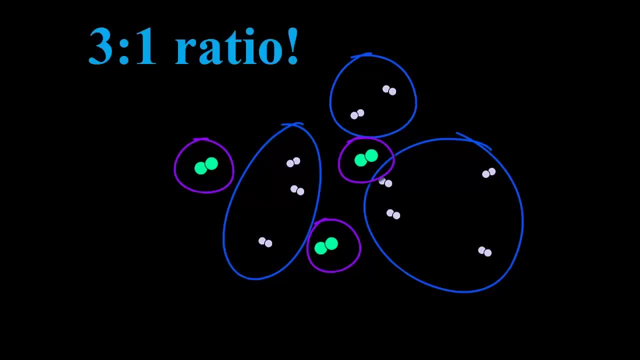 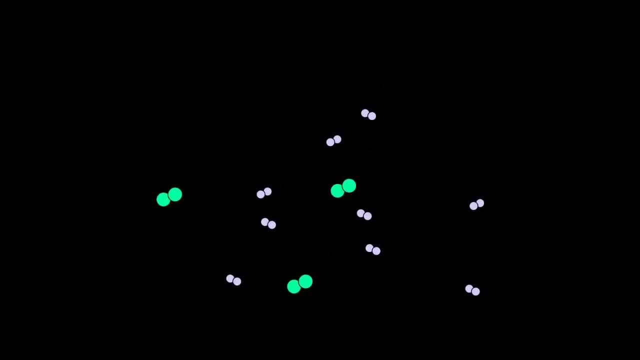 molecules, they're going to react with three nitrogen molecules. So what I'd like you to be able to see here is that, even with larger amounts of molecules, this reaction still occurs, with a ratio of three hydrogens to one nitrogen, producing two ammonia molecules, And with this particular reaction it will always. 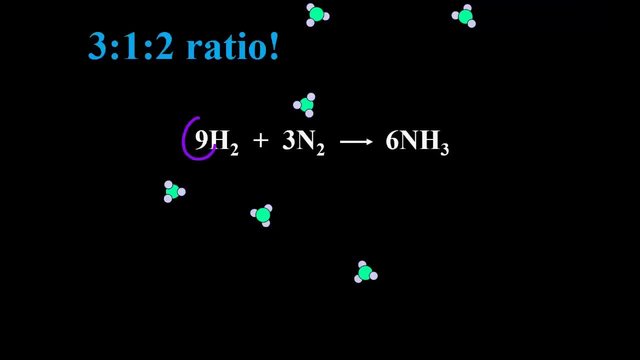 react in that three to one to two ratio. no matter how many molecules you have, You can see we have produced, using nine hydrogens and three nitrogens, a total of six ammonia molecules. Let's back up a little bit and look at what we have here. 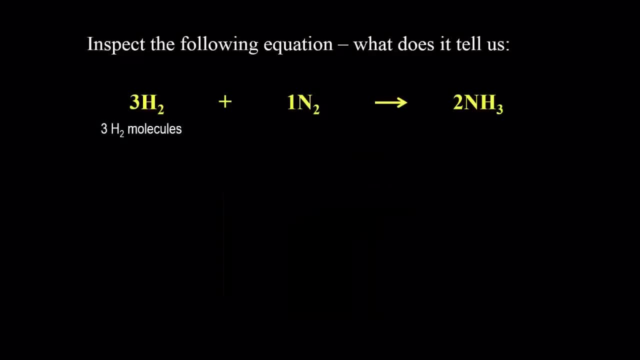 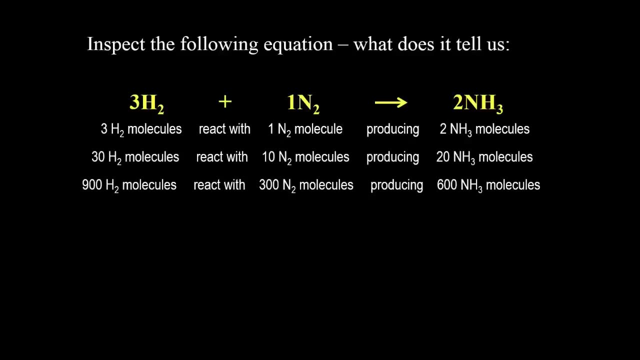 Let's back up a little bit and look at what we have here. Let's back up just a moment. So what's really going on here? Three hydrogens reacting with one nitrogen giving us two ammonia's, but that's really just a ratio. so no matter how many you have, it's always going to be with this reaction in. 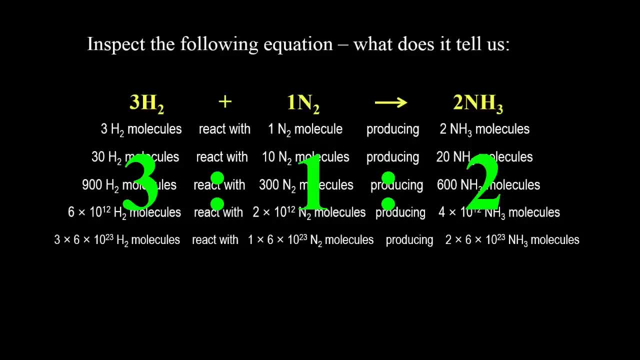 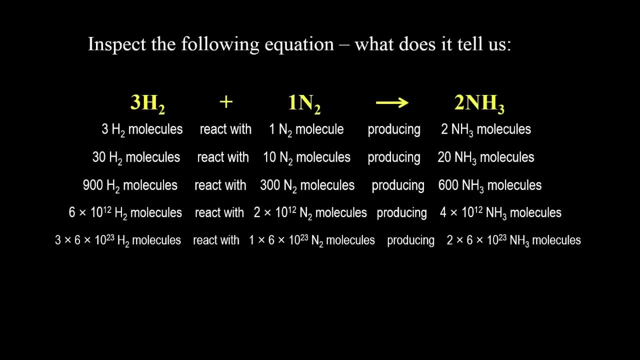 a three to one to two ratio, and so the coefficients of any chemical equation give the ratio of reactants to products in the reaction. The ratios can work for us mathematically because we use the ratio of reactants to products in the imyi will actually use very, very large amounts of molecules at the everyday level. but 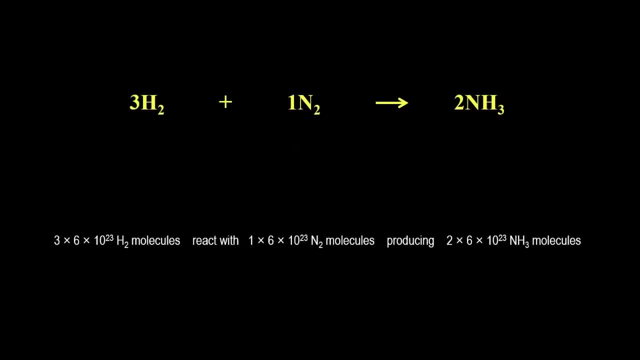 the ratio remains constant. And now we can see how this all connects to molar amounts of particles. Take a look at the last line. We can actually see that the coefficients are molar ratios. We have three moles of hydrogen molecules reacting with one mole of nitrogen molecule and 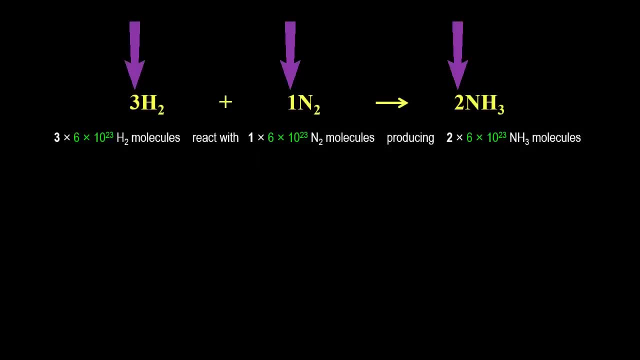 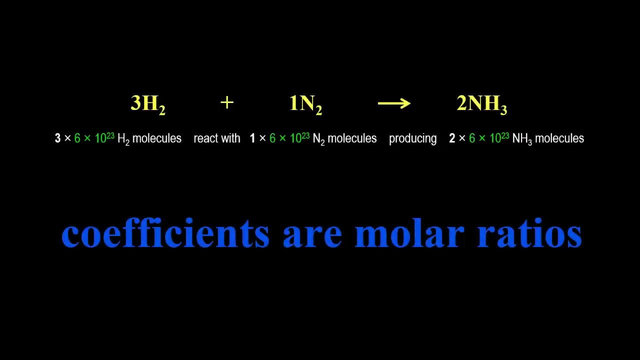 that produces two moles of ammonia molecules. So the coefficients, being ratios, can represent any amounts, including molar amounts, And because we use such large amounts of particles on the level of molar amounts, we use the coefficients as molar ratios. 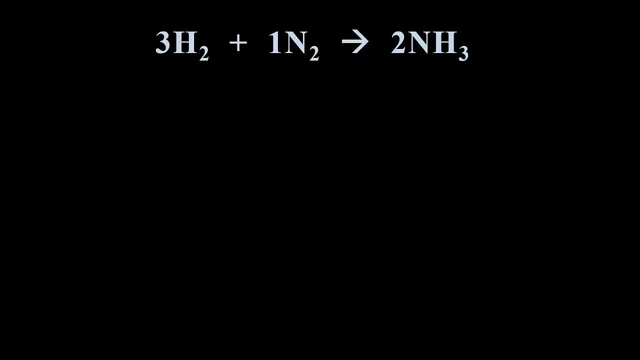 Let's see how that ratio can work for us stoichiometrically. In other words, how can we use that ratio to relate an amount of one substance in a reaction to an amount of any other substance in the same reaction? Keep in mind that the mathematical relationship given by the coefficient ratios hold constant, no matter how much of the substances are being reacted, as we saw in the first part of the video. 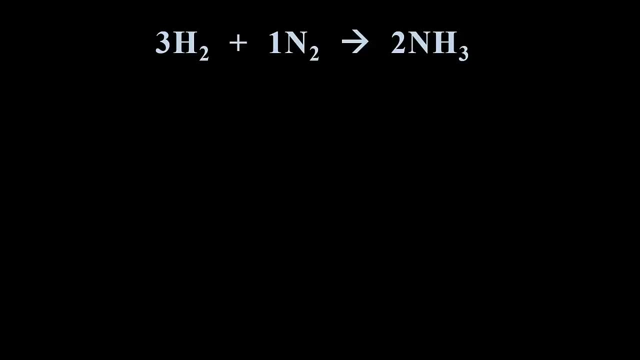 So in the rest of the video we will be looking at various examples to build up to what you might normally see as stoichiometry problems in a textbook. we will look at mole-mole calculations, mass-mass calculations and other stoichiometric calculations. 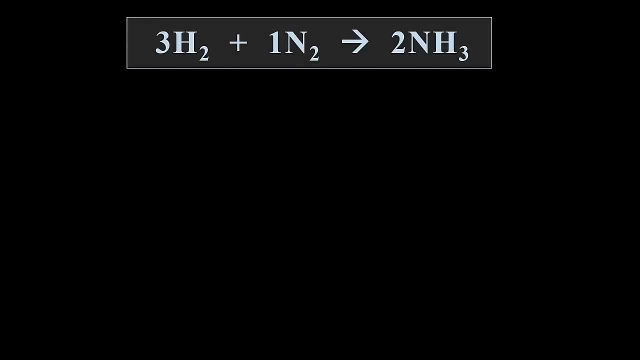 Let's look at an example using this reaction of hydrogen and nitrogen. How many moles of nitrogen are needed to react with 7.5 moles of hydrogen? So if we have 7.5 moles of hydrogen, how many moles of nitrogen would react with that? 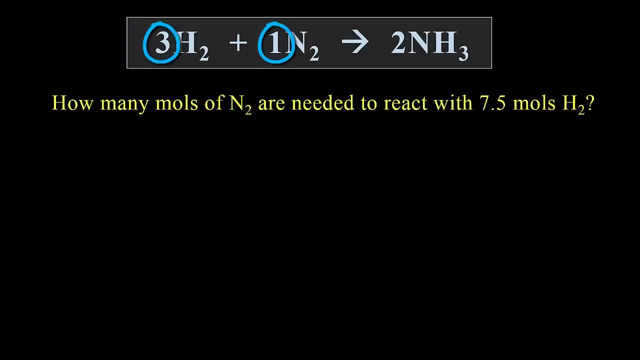 We use the coefficient ratio of three hydrogens to one nitrogen to determine the answer. The amount given in the problem is 7.5 moles, So we have 7.5 moles of hydrogen and we multiply that by a fraction that represents the coefficient ratio. 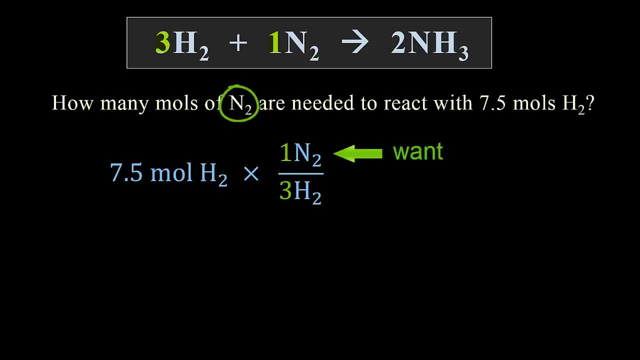 The one nitrogen to three hydrogen ratio, always putting on top what we want and on bottom what we have- tells us that 2.5 moles of N2 will react with 7.5 moles of H2, and 7.5 to 2.5 is a 3 to 1 ratio. 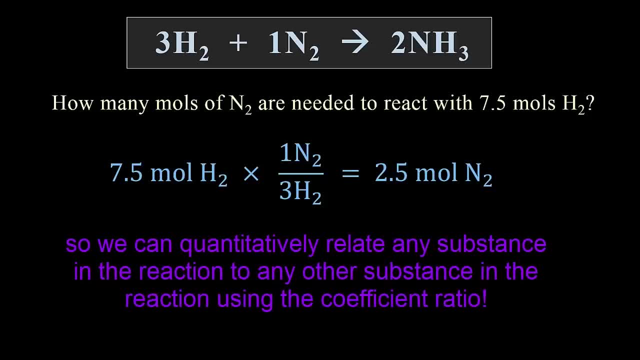 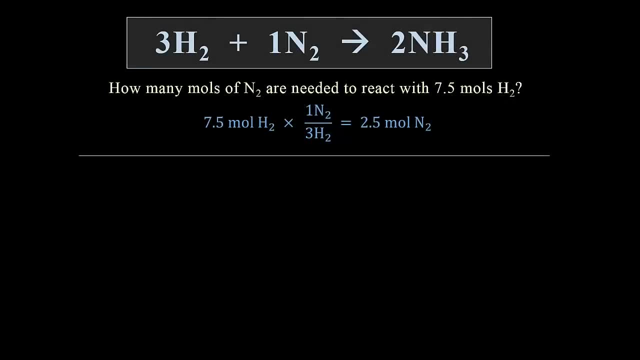 So we can quantitatively relate any substance in the reaction to any other substance in the reaction using the coefficient ratio. Let's look at a second example: How many moles of hydrogen are needed to produce 0.8 moles of NH3?? 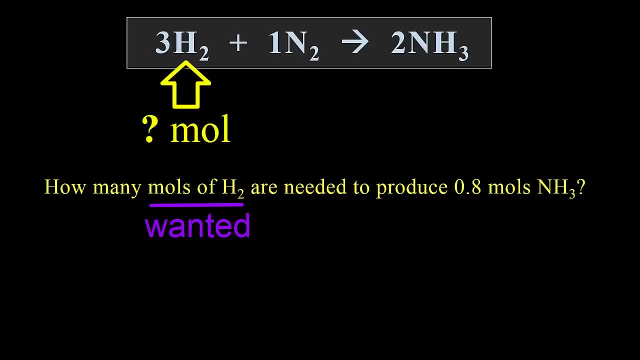 We want to find out how many moles of hydrogen are needed in the reaction to get 0.8 moles of ammonia, NH3.. We write down what's given in the problem- 0.8 moles of NH3, and multiply it by the ratio of three hydrogens for every two NH3.. 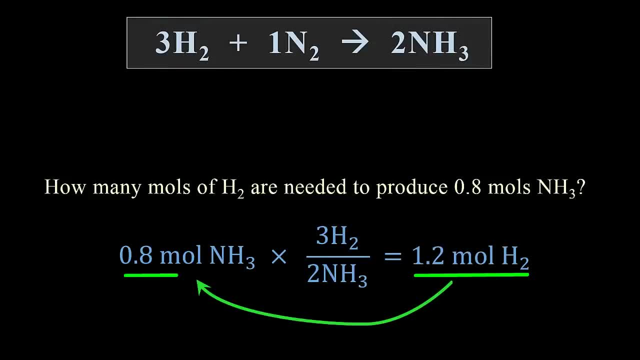 That tells us that 1.5 moles of NH3 is equal to 0.8 moles of NH3.. 0.2 moles of hydrogen are needed to produce 0.8 moles of ammonia In a problem like this, where the other reactant, in this case nitrogen, is not mentioned. 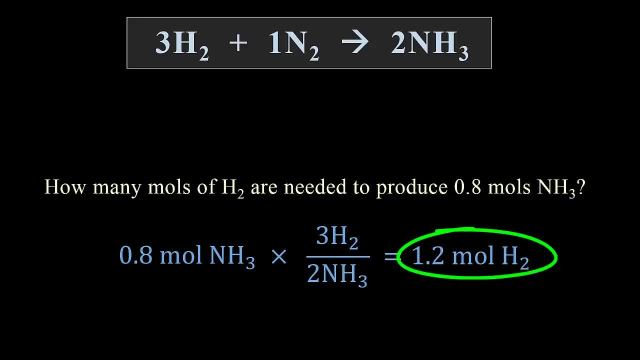 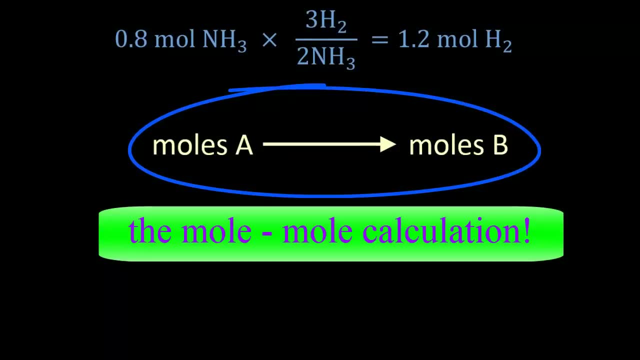 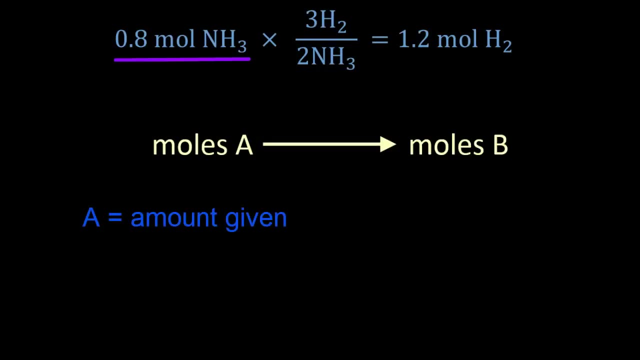 we would just assume that there is enough nitrogen to react with that amount of hydrogen. So this is always the central part of the stoichiometric calculation, the mole-mole conversion. These mole-mole connections always follow the same format, where A is the amount given in the problem. 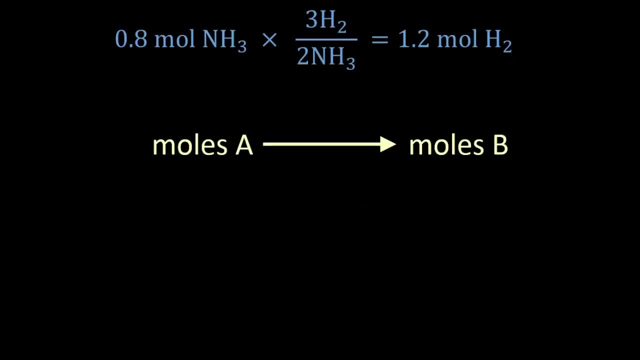 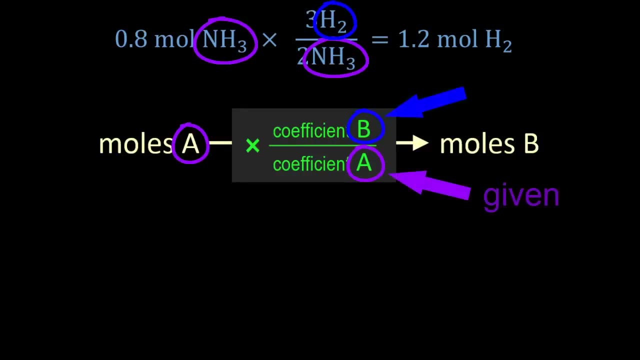 and B is the amount wanted in the problem And multiplying by the coefficient ratio gets us from moles of A to moles of B, the moles given to the moles wanted. Again, this is always going to be the central calculation for any stoichiometry problem. 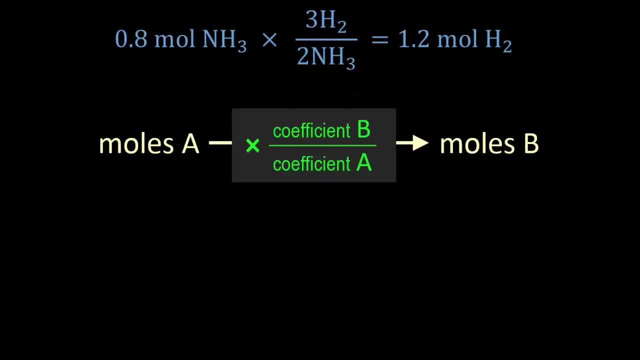 keeping in mind that A- what you start with- goes on the bottom so that it cancels out, and B goes on top so that you end up with what you want. But there is a problem with this: We cannot really know directly the amount of moles. 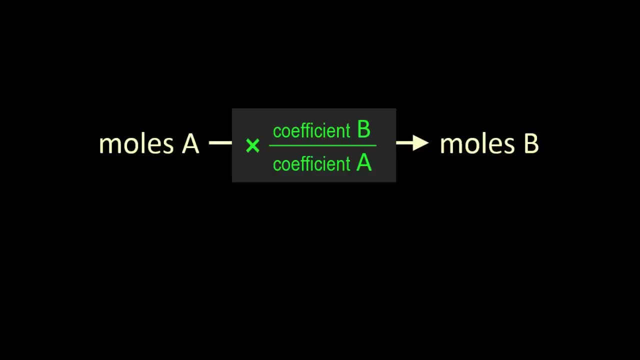 because we cannot count out an amount of particles, But we can weigh amounts of substances which we can then convert to moles. So that expands our map like this: Here is our ever-present mole conversion and given a mass of one substance in the reaction, 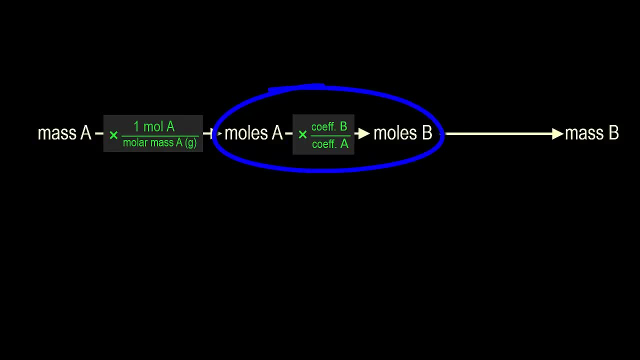 you can convert it to moles using molar mass and then convert to moles wanted and finally convert moles wanted to mass wanted using B's molar mass. We will now see how this map can guide us in a mass-to-mass stoichiometry problem. 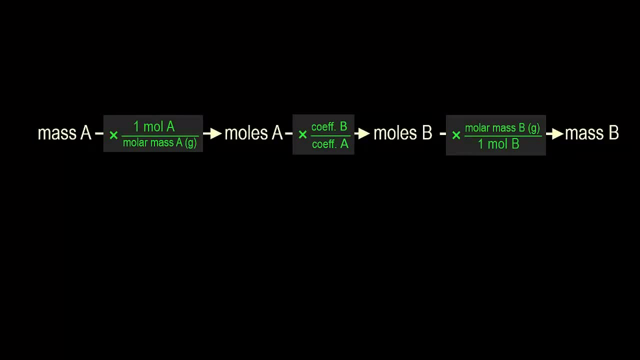 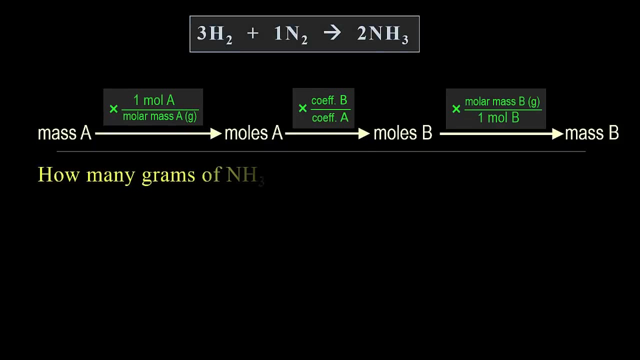 that involves multiple unit conversions. The setup uses the same structure as any dimensional analysis problem. Let's go back to the ammonia reaction. What mass of NH3 will be produced from 42 grams of N2 reacting completely? Let's fill in the map to fit our problem. 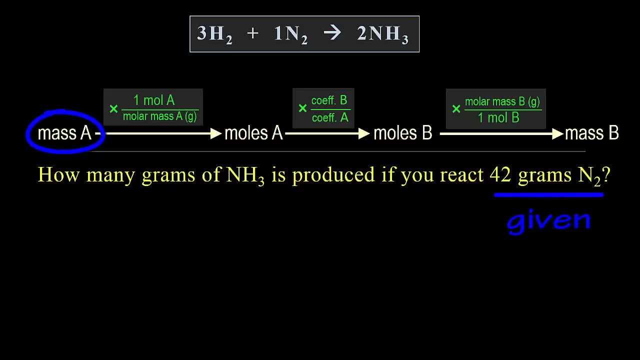 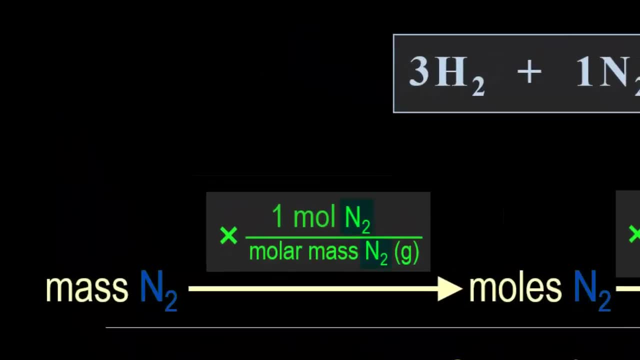 We start with a mass of nitrogen- that's our given- and want to end up with some mass of ammonia, which is the substance wanted. We can see that we first have to convert mass of N2 to moles of N2 using nitrogen's molar mass from the periodic table. 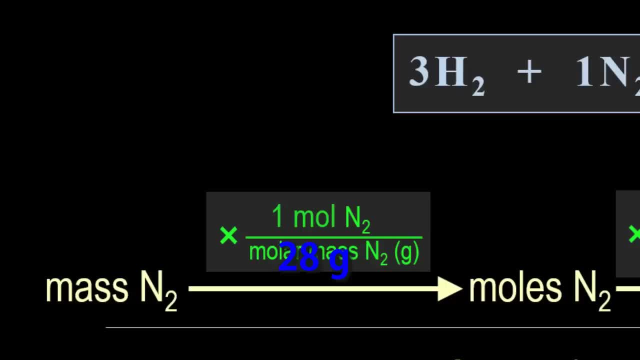 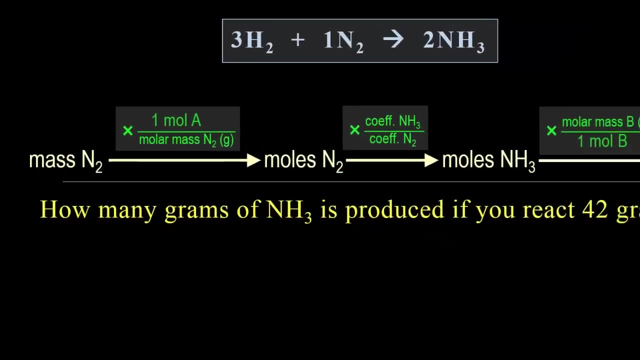 which is 28 grams of N2 in one mole of N2, then moles of N2 to moles of NH3 using the coefficient ratio, and finally from moles of NH3 to mass of NH3 using the molar mass of NH3 from the periodic table. 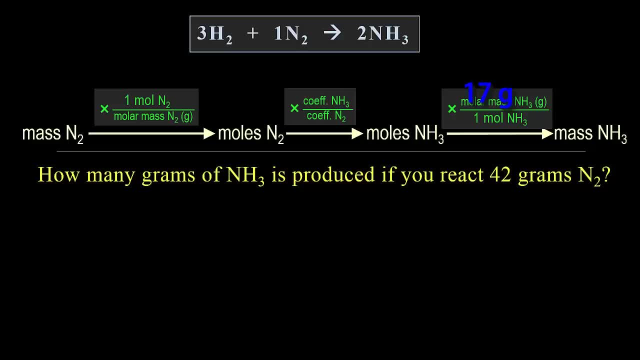 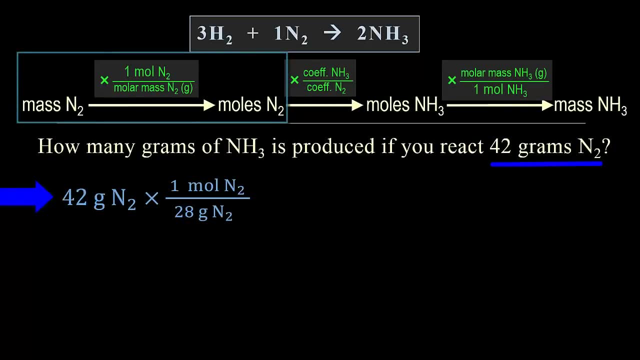 which is 17 grams of NH3 in one mole of NH3.. The amount of nitrogen given is 42 grams, so we multiply that by one mole of nitrogen per 28 grams of nitrogen, This calculation gives us 1.5 moles of N2.. 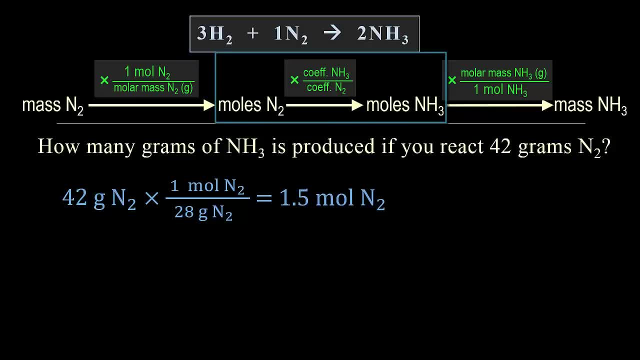 The next step is converting moles of N2 to moles of NH3.. So here's the central part of any stoichiometric calculation: converting moles of one substance to moles of another substance using the coefficient ratio. The last step converts moles of ammonia. 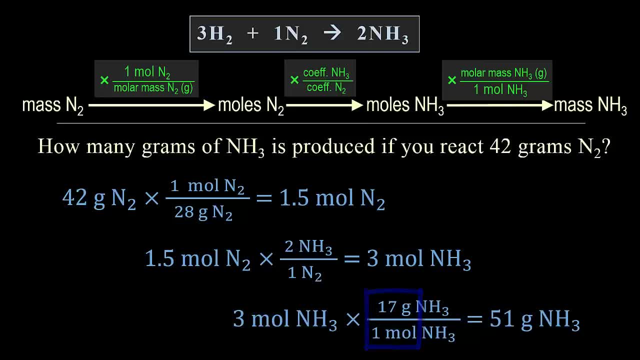 to mass of ammonia using the molar mass of ammonia. So 51 grams of NH3 will be produced from the complete reaction of 42 grams of N2.. Normally with stoichiometry, as in dimensional analysis in general, we can more efficiently write the calculations in a chain. 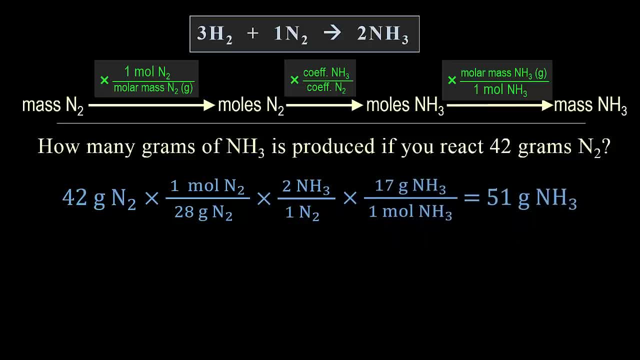 And you can see, as in any correctly written dimensional analysis, all unwanted units cancel and the wanted unit is the one you are left with. If the units don't cancel, you are setting it up incorrectly and will get an incorrect answer. so you will need to go back and review the conversions. 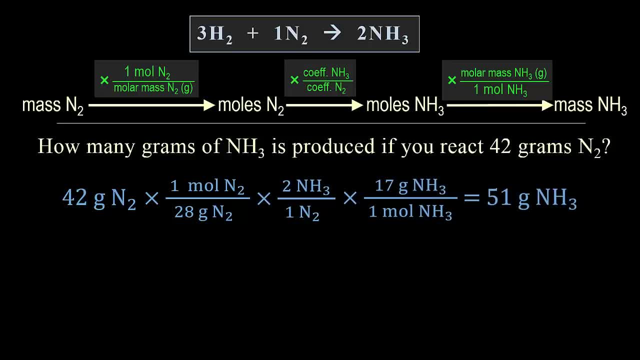 to determine how to fix it. So the steps here are in this chain: This calculation gives us moles of nitrogen, the next gives us moles of NH3, and finally the mass of NH3.. Once it is set up correctly, what you are putting in your calculator. 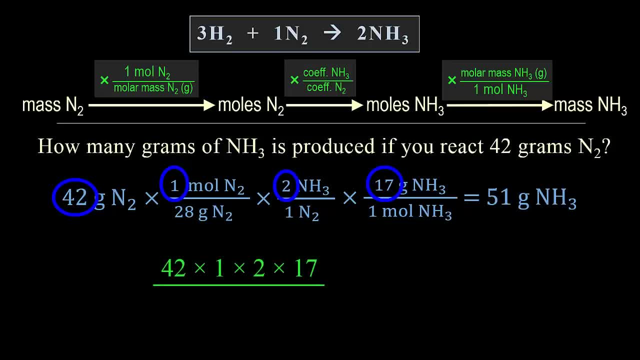 is simply multiplying all the numbers in the numerator and dividing by everything in the denominator. I hope you can see the usefulness of stoichiometry here. A straightforward way for the chemist to determine how much product will form in a reaction or how much of one reactant is needed. 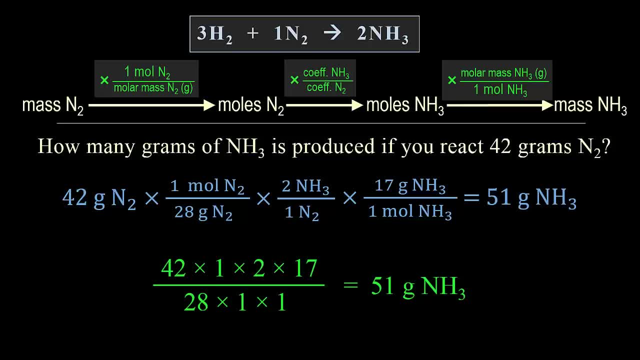 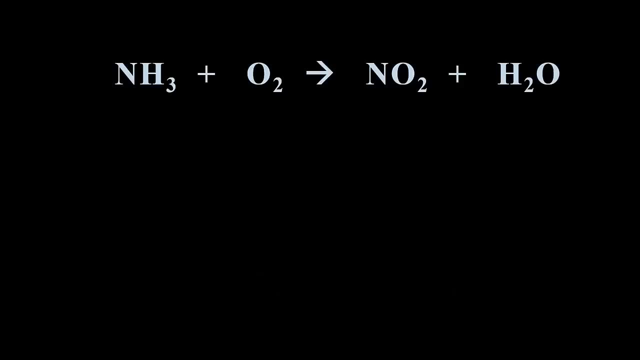 to react with some quantity of the other reactant. We'll do a couple more practice problems and then see how we can extend stoichiometry beyond these mass-to-mass calculations that we are doing now. Here's the next equation: We cannot do stoichiometry without coefficients. 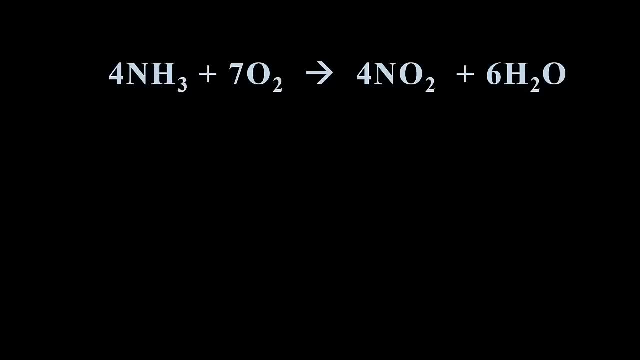 and so we will need to balance Again. these coefficients, like in any reaction, are ratios that we can use as the central part of the stoichiometric conversion from moles of one substance in the reaction to moles of some other substance in the reaction. 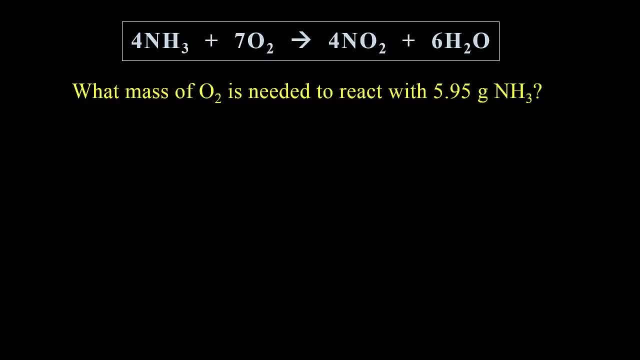 So what mass of O2 is needed to react with 5.95 grams of NH3?? Identify the amount of O2 which is 5.95 grams NH3 and identify what is wanted, which is mass of oxygen. Let's draw a map to guide our chain of equations. 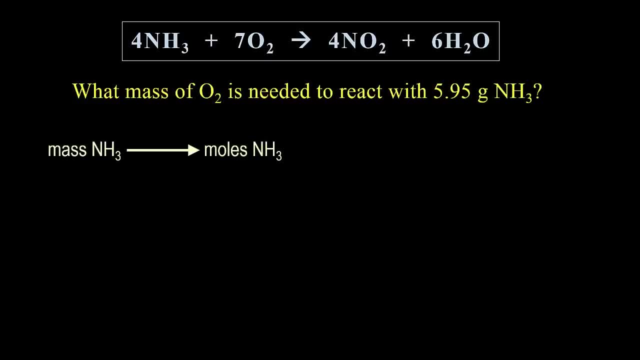 Mass of NH3 to moles of NH3. to moles of oxygen. to mass of oxygen, We have the coefficients from the equation and the molar masses from the periodic table. Starting with 5.95 grams of NH3 convert to moles of NH3. 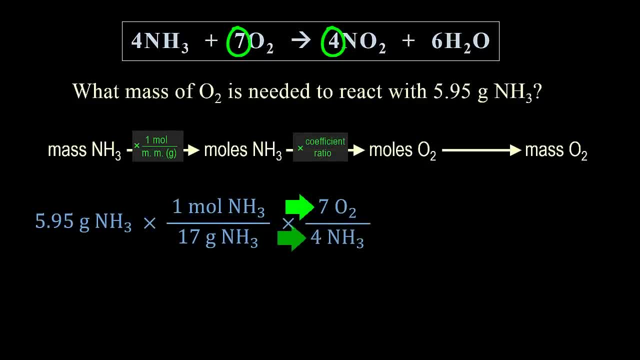 then to moles of NH3 and total to 6.2 grams of oxygen and the SoH of the coefficient ratio, and then to mass of oxygen using the molar mass of oxygen. Make sure everything cancels out so that we are left with mass of oxygen. 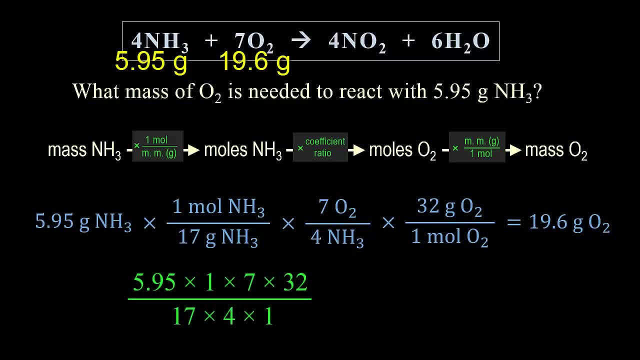 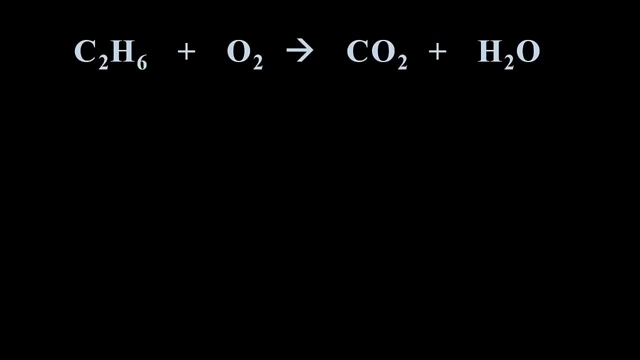 which comes out to 19.6 grams. The calculation is multiplying the numbers on top, dividing by the numbers on bottom. Let's do one more mass-mass practice: the combustion of ethane, C2H6.. First we'll add coefficients to balance What? 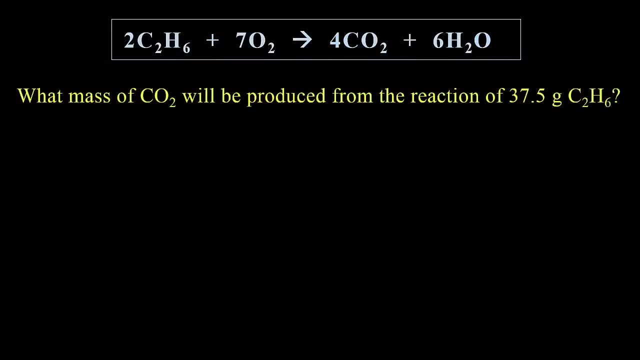 mass of carbon dioxide will be produced from the reaction of 37.5 grams of C2H6?. Why don't you turn off the video and see if you can work it out and then come back to see how you did? If you have trouble getting started, let's first make. 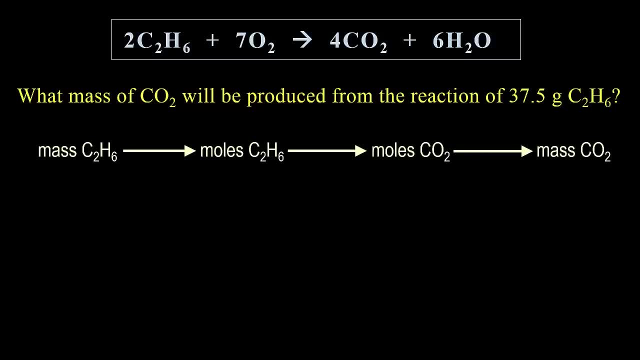 a map and then follow the map. Here is our map. We start with what's given, convert to moles, then the mole-mole conversion, then convert to mass of carbon dioxide. We start with what's given, convert to moles, then the mole-mole. 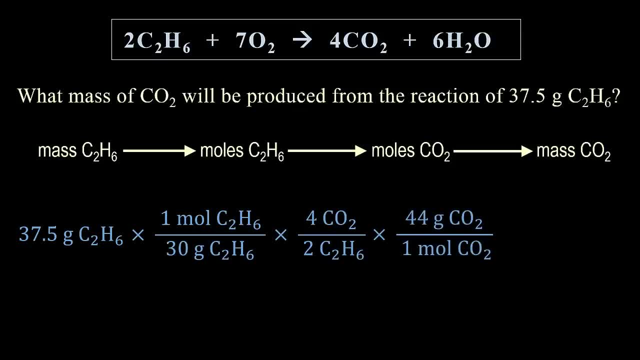 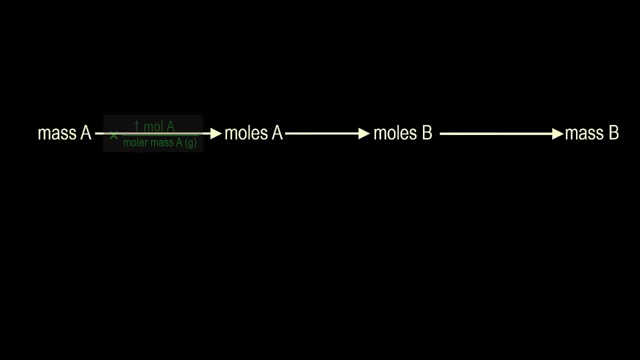 conversion, then convert to mass of carbon dioxide. So the reaction of 37.5 grams of C2H6 produces 110 grams of carbon dioxide. Now let's move on to other types of stoichiometric calculations. The central calculation is always provided by the mole-mole calculation, and so any quantity given 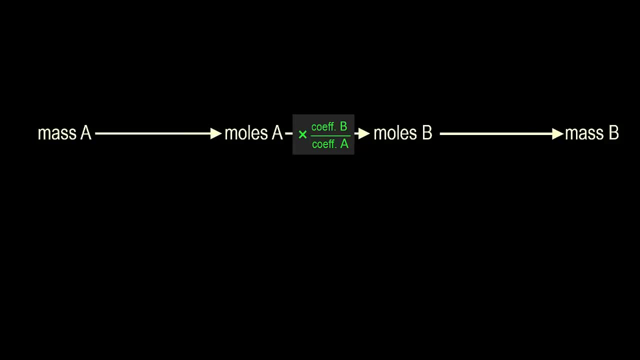 that can be converted to moles can expand the repertoire of calculations. For example, suppose the problem gives some amount of particles in a reaction rather than mass, or wants to end up with particles. Particles refers to atoms, ions, molecules or formula units. These can be converted to moles and from moles using 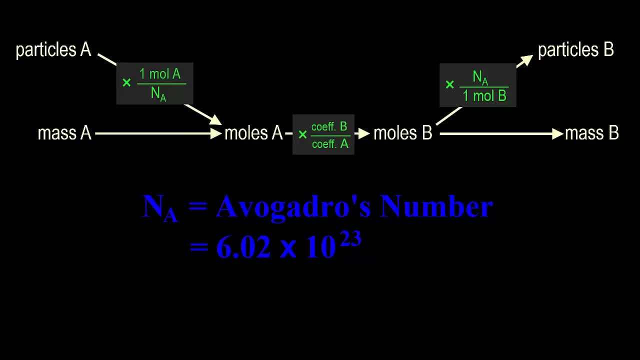 Avogadro's number 6.02 times 10 to the 23rd, Because one mole of particles is equal to 6.02 times 10 to the 23 particles. Similarly, if you are working with volumes of gases in the equation at, 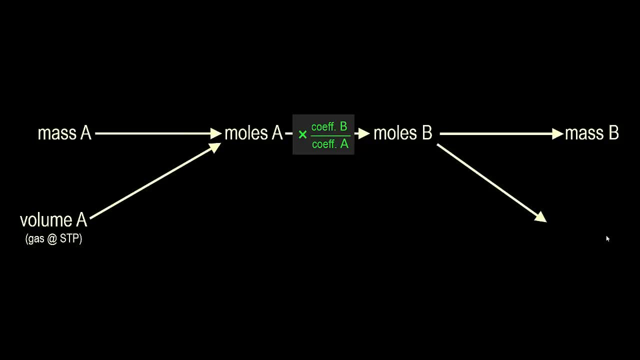 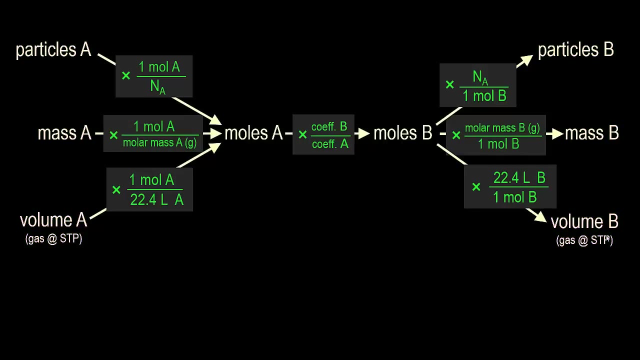 standard temperature and pressure. you can use the fact that a mole of gas particles occupies 22.4 liters at STP. So now we can see the map giving us the path to convert to or from particles mass or gas volume. For example, a problem that gives us gas volume and asks for particles would first convert.